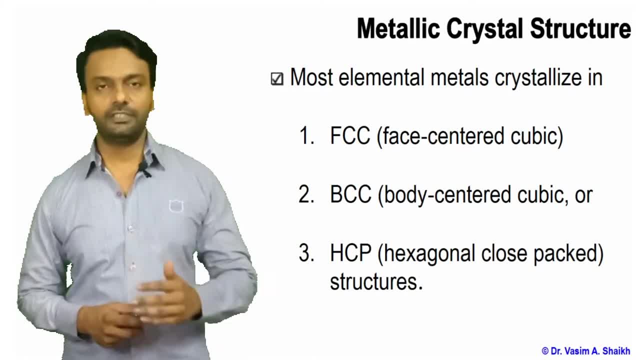 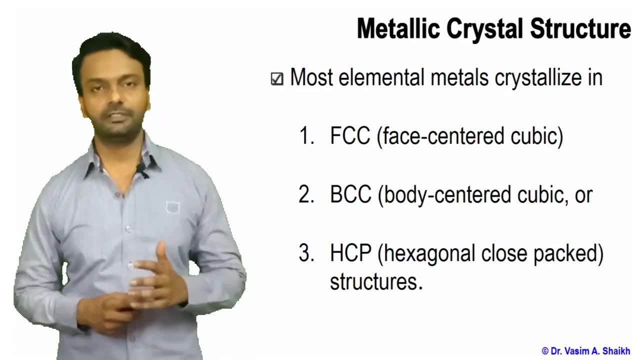 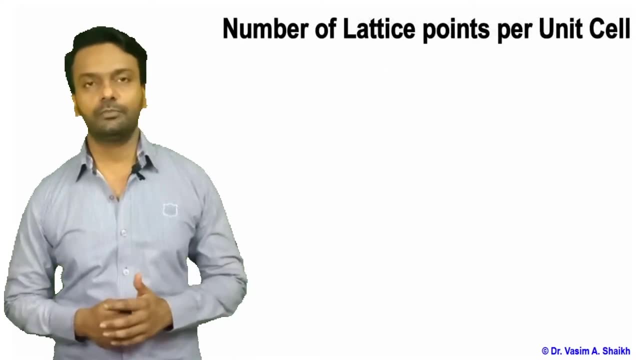 So now let us see each one of these crystal structures, how the atoms they are located in each and every crystal structure: FCC, BCC and HCP. But before that let us see how we can calculate or how we can know the number of lattice points which are there per unit cell. 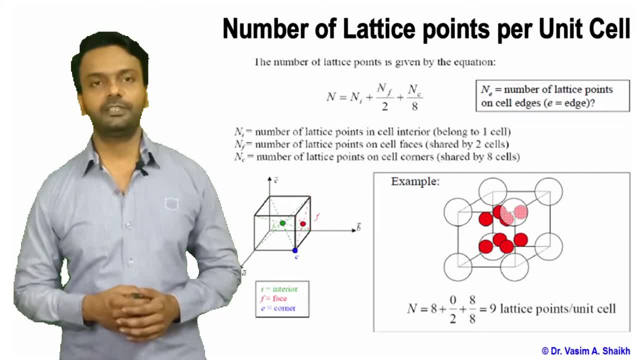 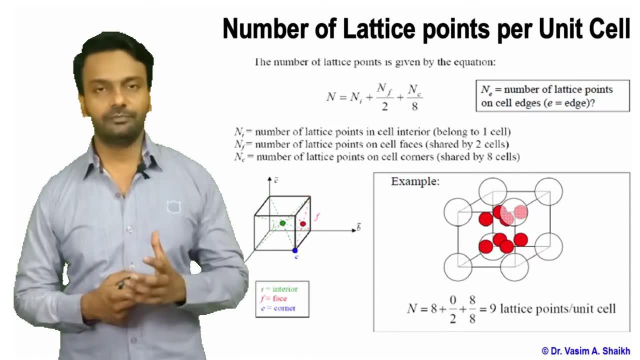 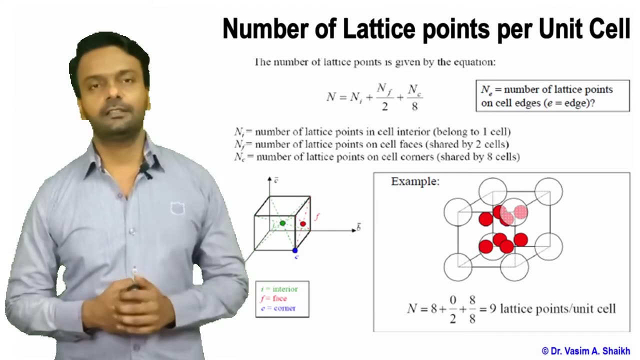 So number of lattice points per unit cell is basically calculated by the formula N. So here the formula N basically shows that if the atom or any point is in the interior, So it is given a subscript INI. That means The atoms are in the interior. 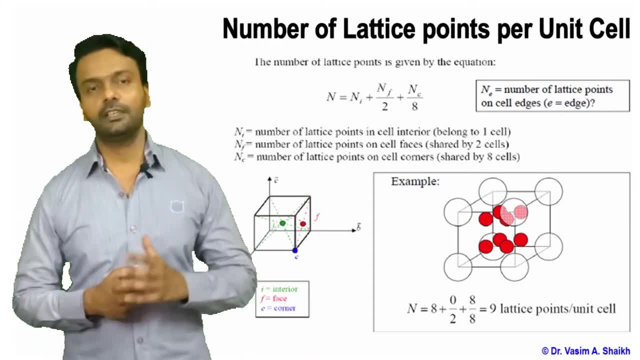 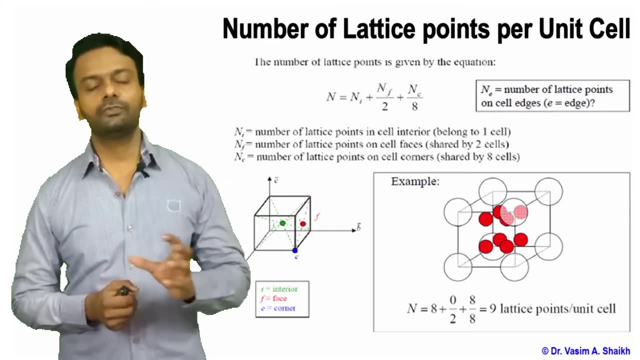 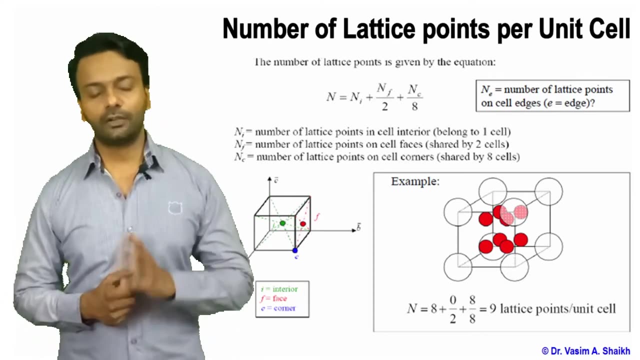 Here, in the below mentioned example, if you see the red atoms or the red lattice points, these are interior, These are internal in the unit cell. So we can count them as one. So we can count them as one. And if suppose the atoms are located on the faces of the unit cell, of the face of the unit cell, then we have to take them as half. 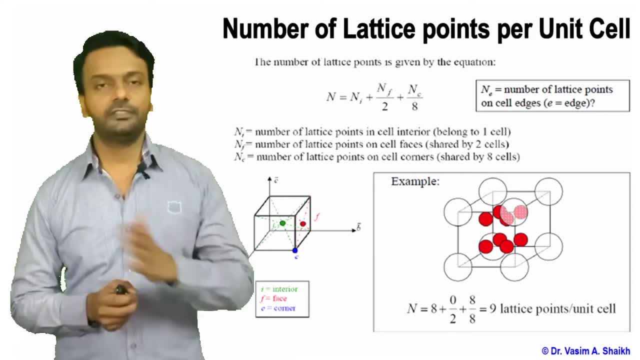 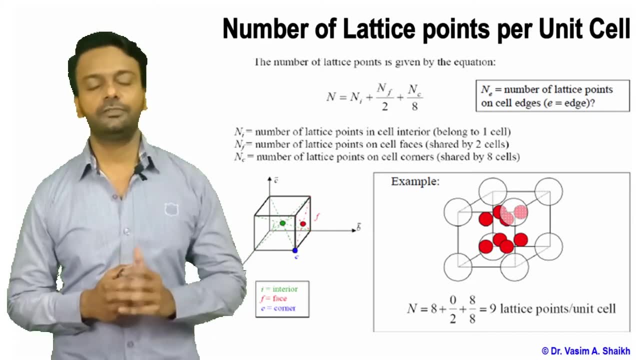 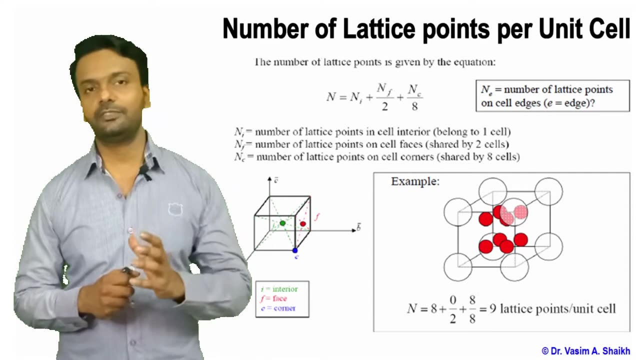 That means half is in one unit cell And half is in the other unit cell- Then if the atoms are located on the corners- So here if you see the unit cell, eight atoms are shown in the corner. That means you have to take such atoms as one eighth. 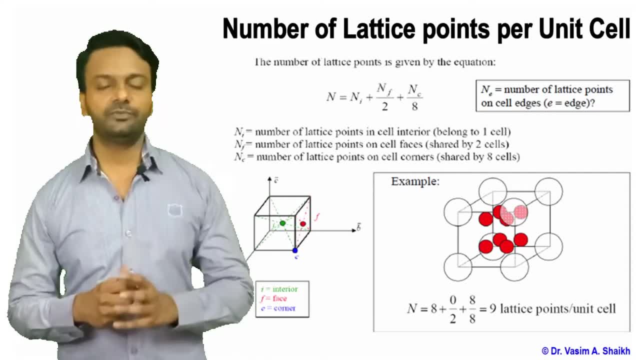 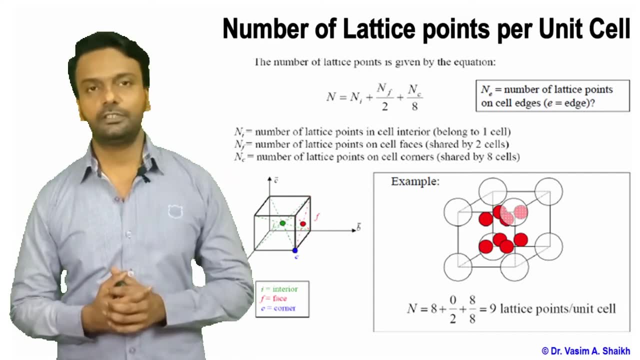 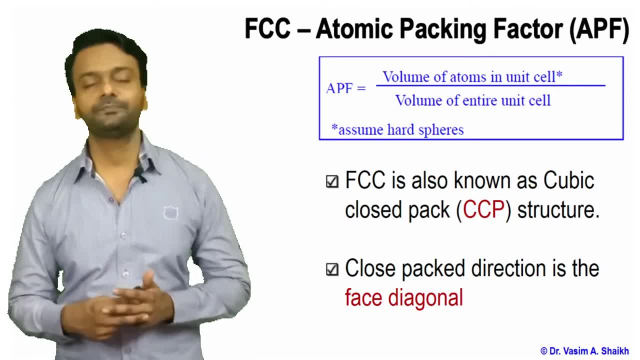 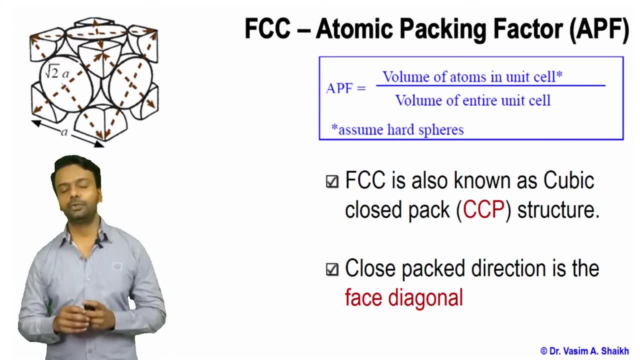 on the phase diagonal of the structure. So here this is a hard sphere model and then you can see: A is the lattice parameter and then root 2A is the phase diagonal, and root 2A means A is the lattice parameter. that can also be equated to 4R, that means the radii of the atom, and that is the 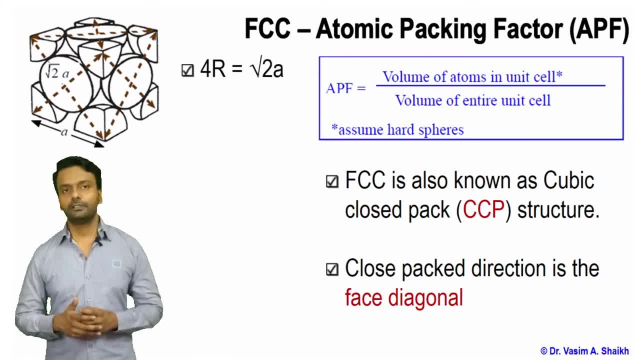 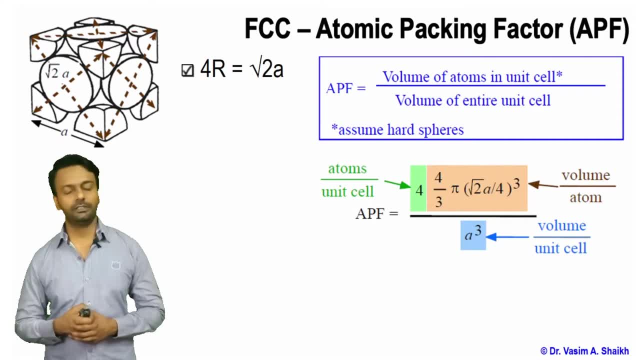 equation which is shown there. Now let us calculate the atomic packing factor, So APF, so volume of the atoms in the unit cell. So first of all we should know how many atoms are there in the unit cell. Then we have to multiply that number of atoms with the volume, volume of the 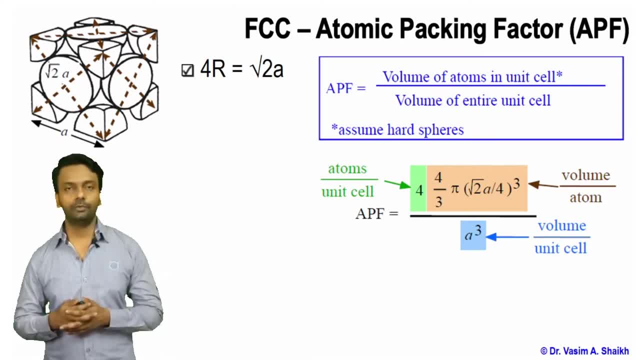 sphere over A cube is nothing but the volume of the cube. So how we got 4?. Now let us see how we got 4.. So let us see how we got 4.. So let us see how we got 4.. So let us see how we got. 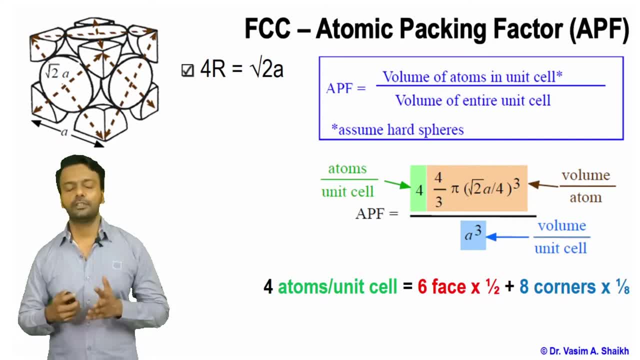 that four, four atoms per unit cell. so we know that in a face centered cubic we have six faces and six atoms are located on the faces. so half is inside, half is outside. so here, if we equate that, we get three atoms, three atoms on the faces and 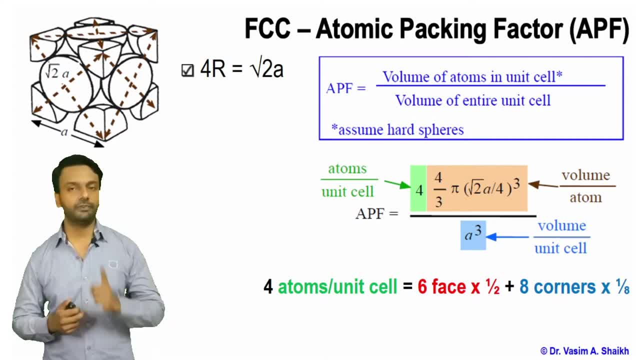 eight corner atoms. so 1, 8. that means one item in the corner. so 3 plus 1 we get four atoms per unit cell in a face centered cubic structure. so we insert that 4 in the equation. so 4 multiplied by 4 by 3 pi r cube, here 4 by 3 pi r cube. 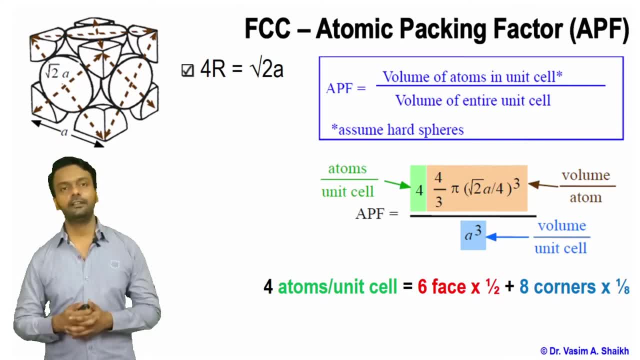 is nothing but the volume of the sphere. okay, and r cube is the radii of the atom that we are equating and we are shown in the top. that is root 2a and that is how we are getting the entire equation and then the atomic packing factor, if we 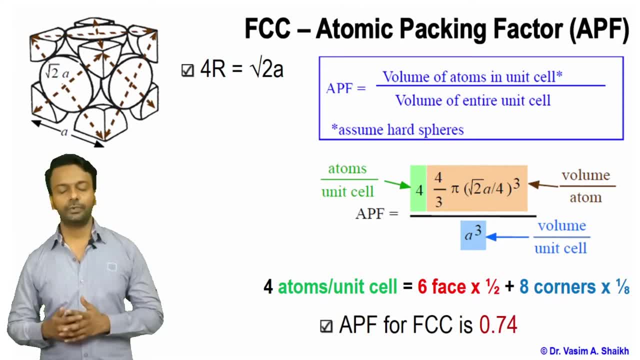 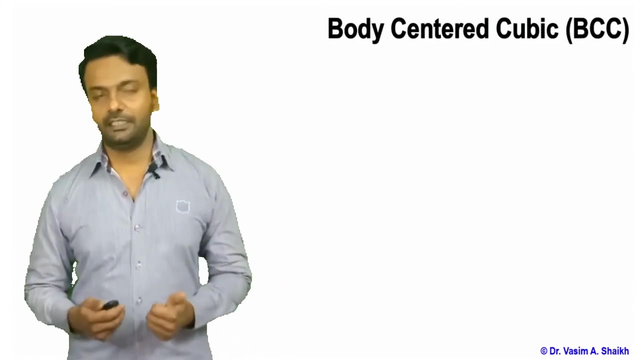 calculate it comes out to be 0.74. that means the atoms are packed 74 percent. the unit cell of a face centered cubic is packed around 74 percent. so this 26 percent is empty space in the unit cell of FCC. so now let us move on to body centered cubic, BCC, body centered cubic. so atoms: 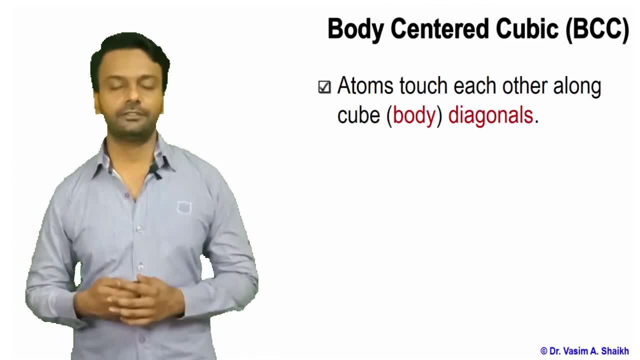 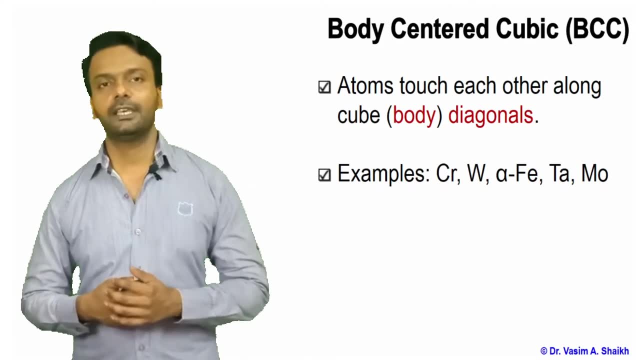 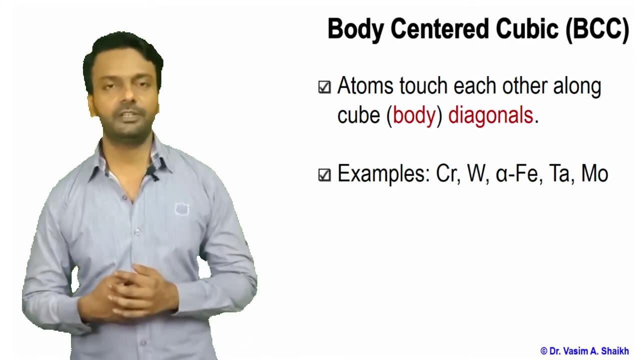 touch each other at the body diagonal. so in the body diagonal the atoms are touching each other- heart sphere. model of body centered cubic. example of bcc structure is chromium, tungsten, alpha, ferrite, tantalum, molybdenum. lot of different elements are there which crystallizes in body centered cubic. 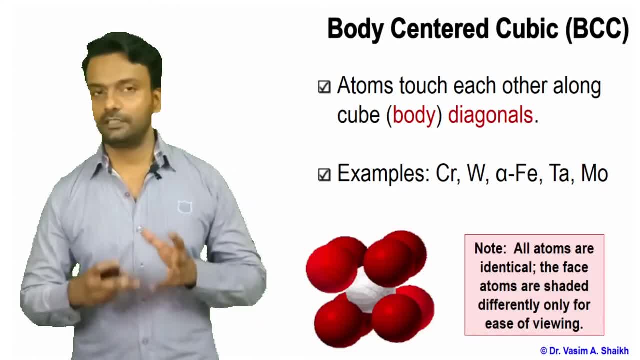 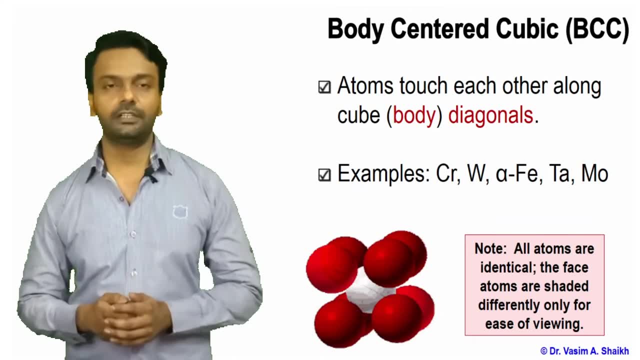 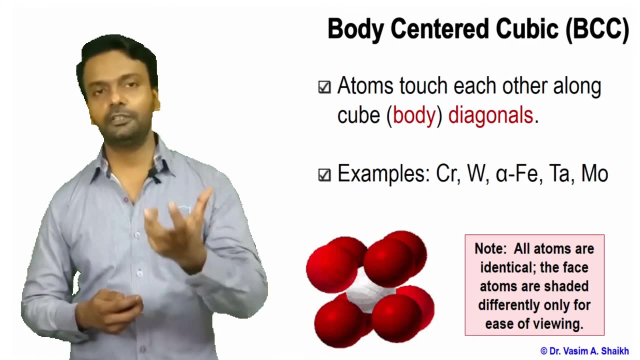 structure. so this is the heart sphere model, again silver color and red color, but the atoms are same. just for our understanding, we are showing that in different color. so here one atom that is silver. it is located exactly in the center. that is why it is called as body centered cubic and eight atoms. 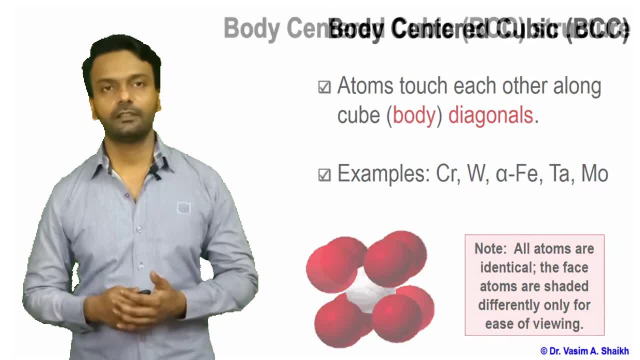 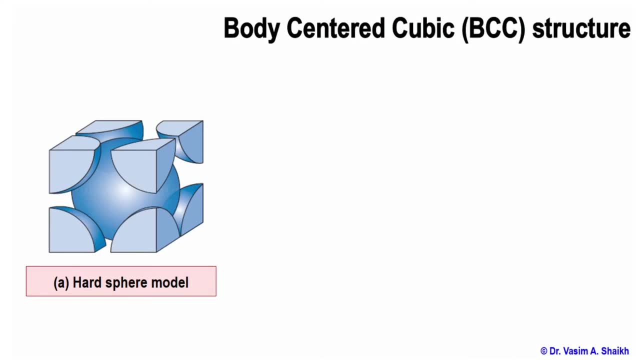 are located on the edges now in body centered cubic. this is a heart sphere model. in actuality, as we have seen, the atoms are touching each other at body diagonal. that is the heart sphere model, reduced sphere model. that is for our understanding. we can understand that. you know. this is how the 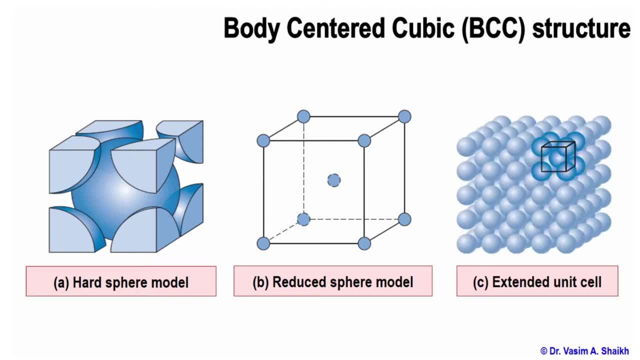 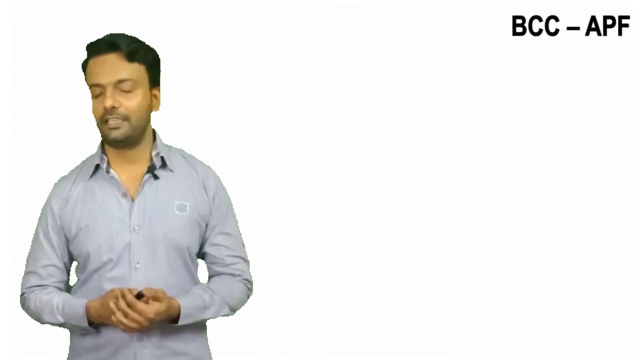 atoms are located and extended sphere model or extended model here. if we have a single crystal of bcc structure, it will grow exactly like this: each and every unit cell has the same orientation as the neighbor unit cell. then let us calculate the atomic packing factor of bcc. same formula we. 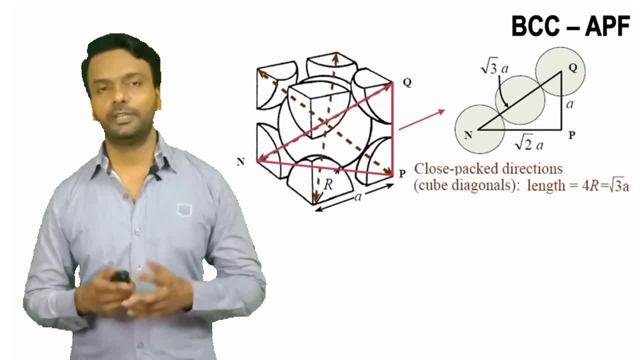 have to apply and same thing we have to do, but here the calculations are different in terms of that. now the body diagonal is different, so the formula comes out to be like this: that 4r is equal to root 3a. this time, 4r is equal to root 3a, and this is the atomic packing factor of bcc. 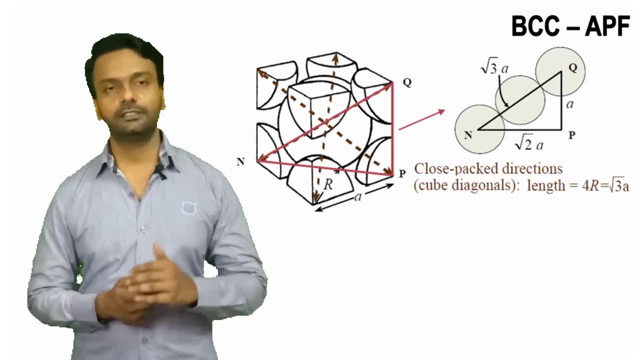 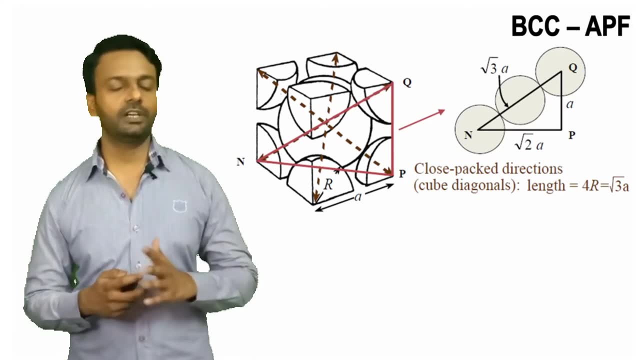 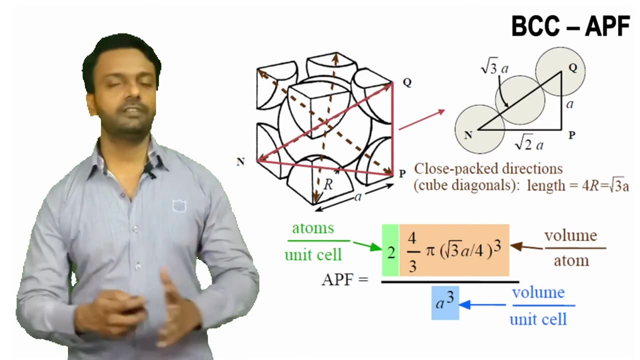 to root 3a because the body diagonal is a closed packed plane. and then we have to take the body diagonal, not the phase diagonal. Initially for calculating 4r we were taking phase diagonal for FCC but here body diagonal for BCC. Then again we put the same the values in the same formula. 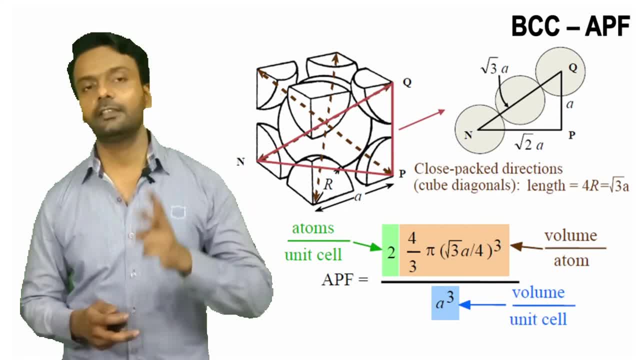 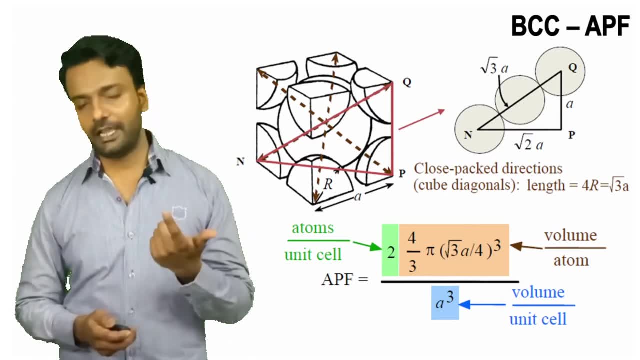 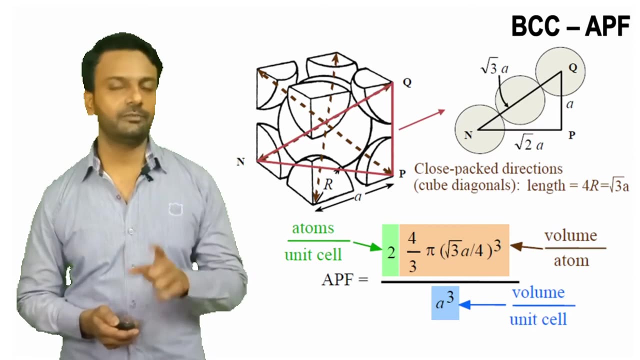 for calculating the atomic packing factor. Here we are getting two atoms per unit cell, So one atom is in the interior. so that is one atom, and eight atoms are at the corner. so we have 1, 8 over 1, 8 into 8. that means 1.. So 1 plus 1 is equal to 2, and then we get two atoms per unit cell. So here 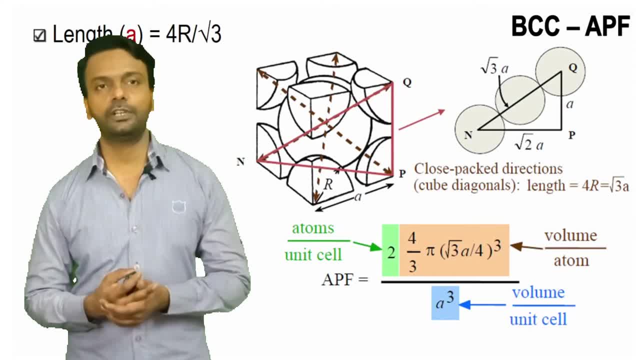 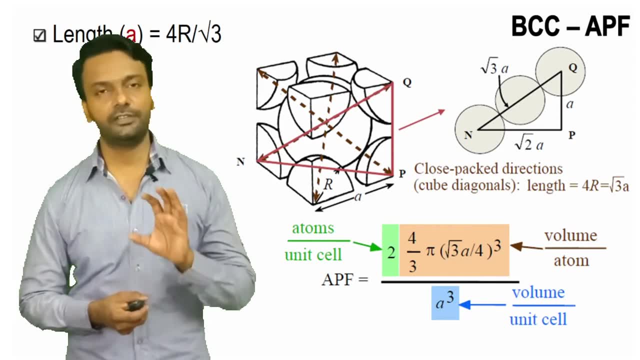 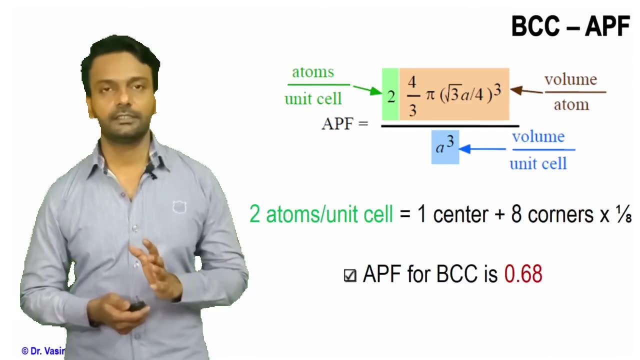 the length a, we got it as 4r over root 3. that is how we are calculating. We insert that value in the volume of the sphere and we get the entire 3r. that comes out to be 0.68.. So 2 atoms per unit cell, 1 in the center, 8 in the corner. So 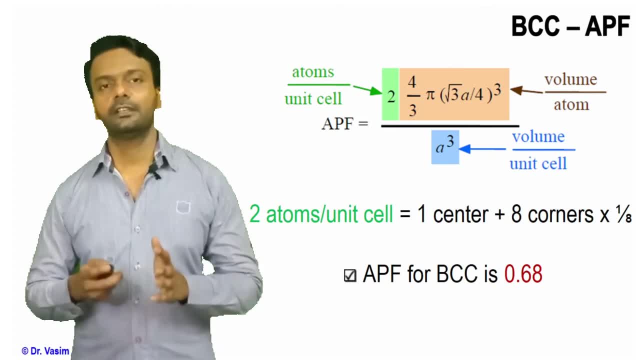 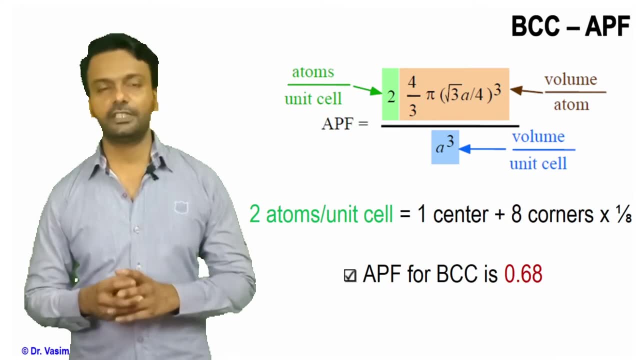 1 plus 1 is equal to 2, 2 atoms and the answer comes out to be: the atomic packing factor comes out to be 0.68.. That means 68% of the unit cell is filled with atoms and rest is completely empty. 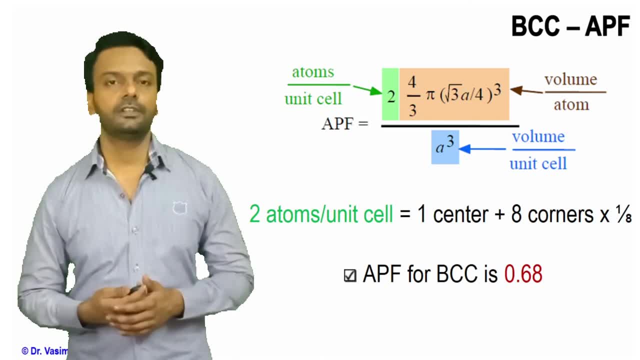 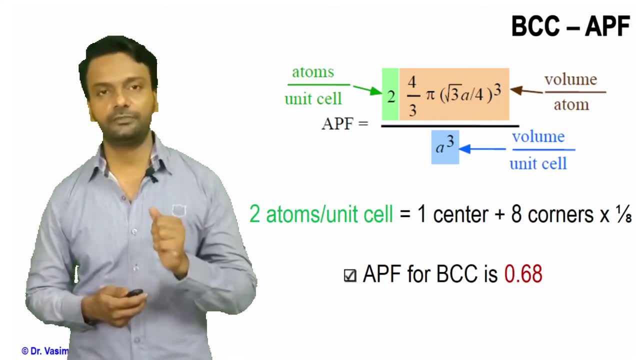 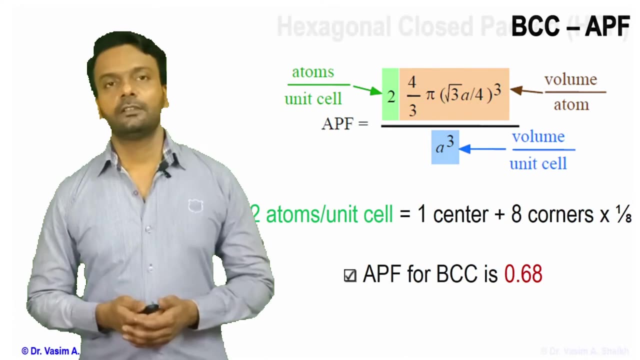 That is how we assume that. you know, there is more space for the interstitial atom to go in VCC structure rather than face centered, cubic or FCC, because the packing factor there is 74,. the packing factor here is 68%. Okay, Now let us move on to hexagonal closed pack or HCP structure. 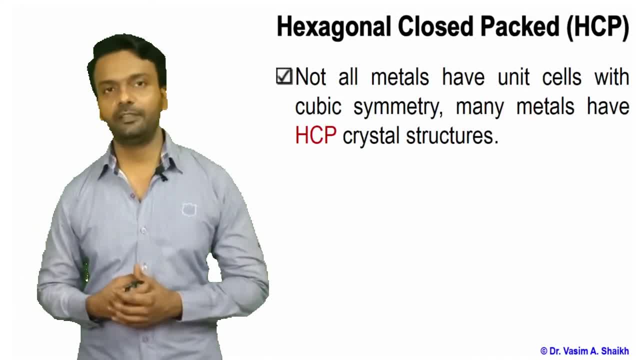 So not all metals have unit cell with cubic symmetry. Many have the HCP crystal structure as well. That is the HCP structure. So that is the HCP structure. So that is the HCP structure. So now let us make it simple. Here is hexagonal closed pack. Examples are zinc, magnesium. 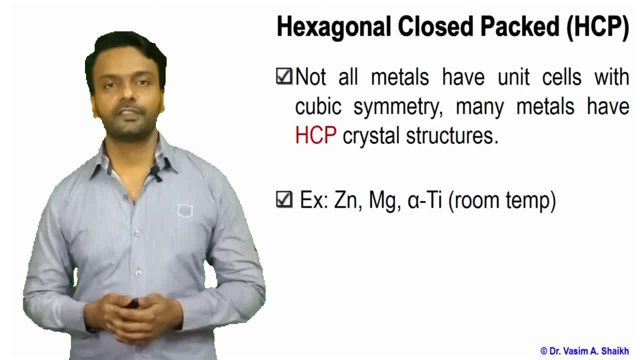 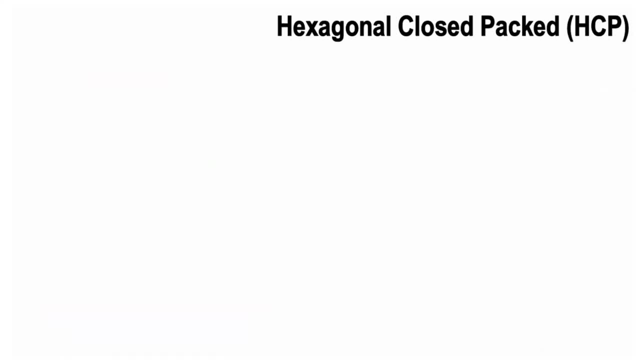 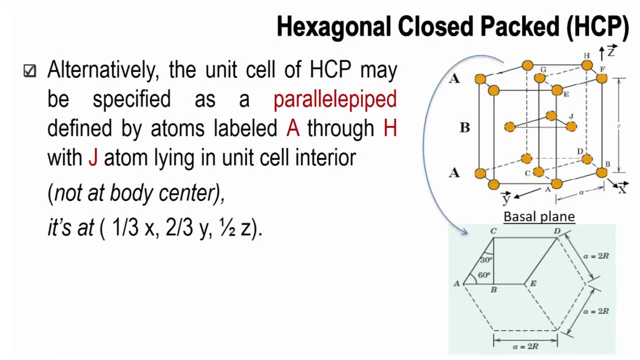 and alpha titanium at room temperature. So these are some of the examples. which crystallizes in a HCP structure. So, alternatively, the HCP structure is also specified as a parallel of pipette. So here you see the image here. This is the HCP crystal. 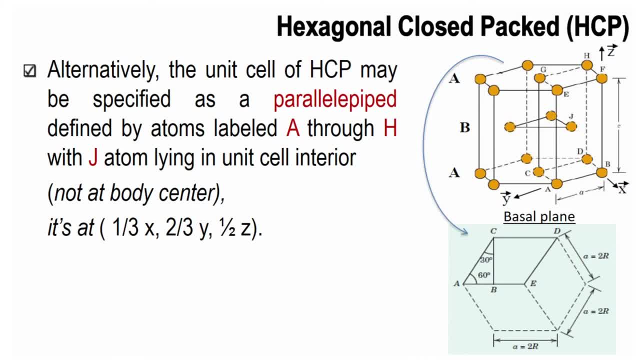 structure and from the atoms which are labeled from A to H. A, B, C, D had done. H and H are the bottom and EFGH at the top. you can see that it is a parallel of pipette, and then we can. 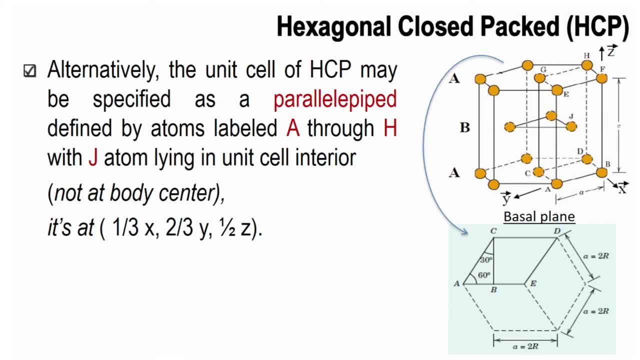 calculate similarly, you know like how, how many atoms are there in the unit cell, and so on and so forth. so if you take that, then atoms are located at one third of x. so you can see x, y and z is shown here: if you take from x, it is one third. if you take from y, it is two third, and then it is. 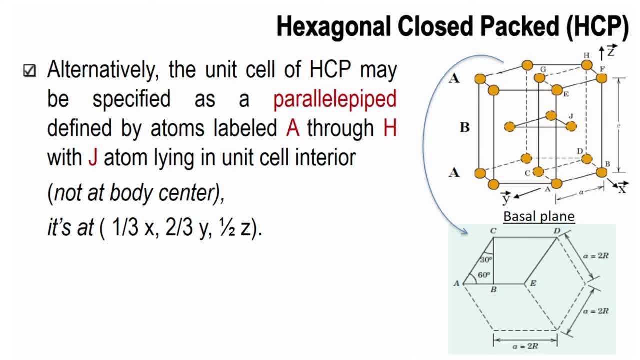 exactly located in the center, so that interior atom- okay, that is the interior and it is not in the body center, it is an interior atom and that is the location of the atom, that it is in the interior and it is one third x, two third y and half of z, the basal plane which is on the top. 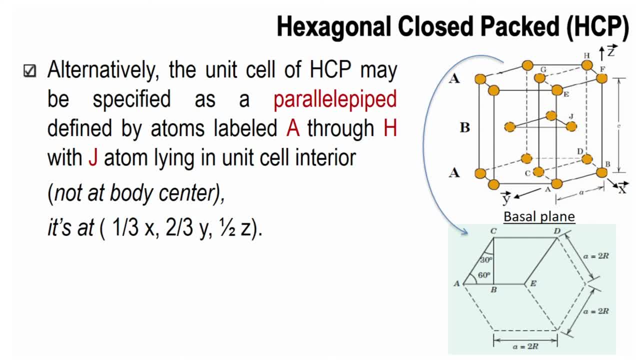 the top plane is shown here in the bottom image. that, that is the top view of that particular plane, is shown at the bottom, and you can see that a is equal to 2r, and then this is the extended cell which is shown here. and finally we can calculate that there are eight- sorry six- atoms in a unit cell of a. 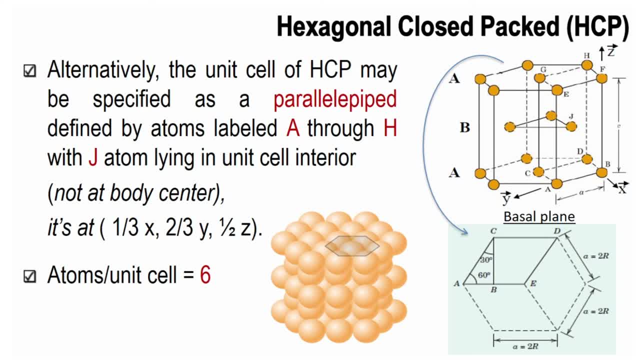 hcb structure: three plus one plus two is equal to six. so six atoms are there, three interior, one on the basal plane and two in the corner or in the edges. so that comes out to be six atoms per unit cell. and the atomic packing factor: if we count it comes out to be 0.74. 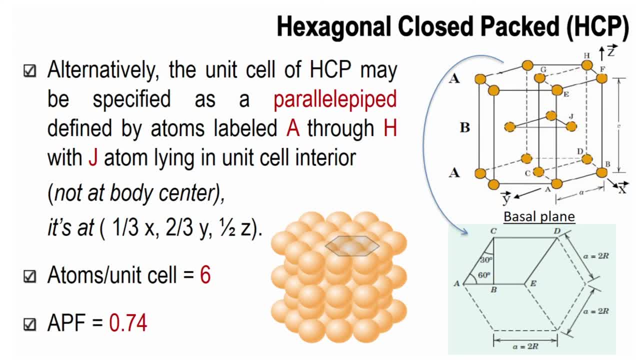 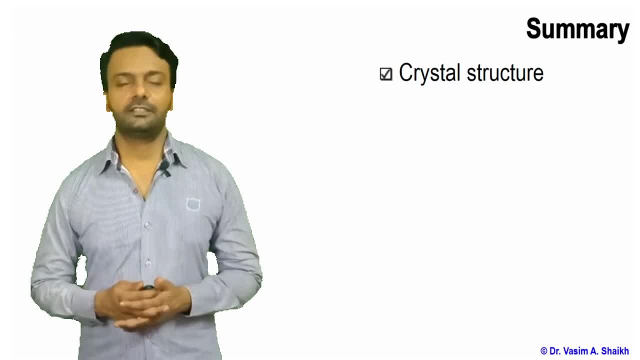 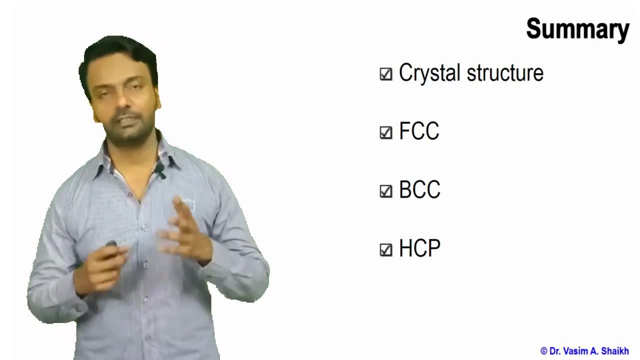 similarly to or same as the fcc crystal structure. so let us summarize what we have studied today. we saw fcc crystal structure, and then we saw bcc, and then we saw hcp crystal structure, fc crystal structure. basically, the six atoms are there on the faces. 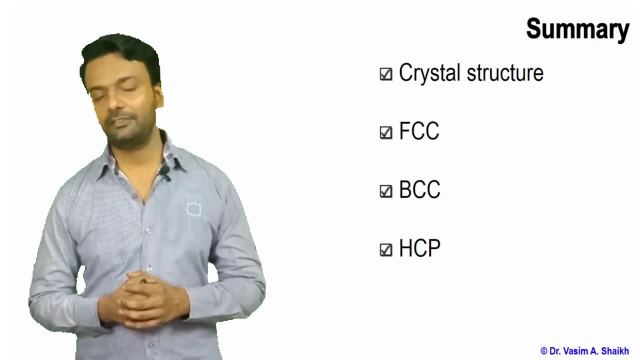 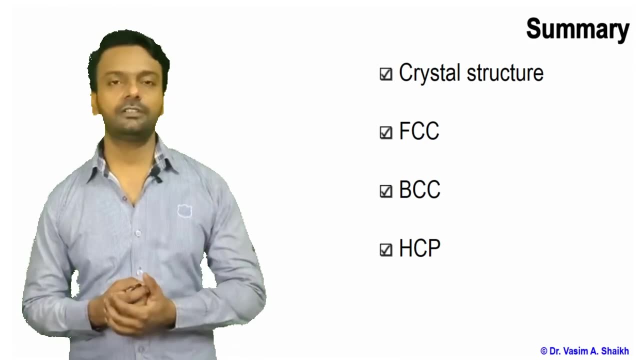 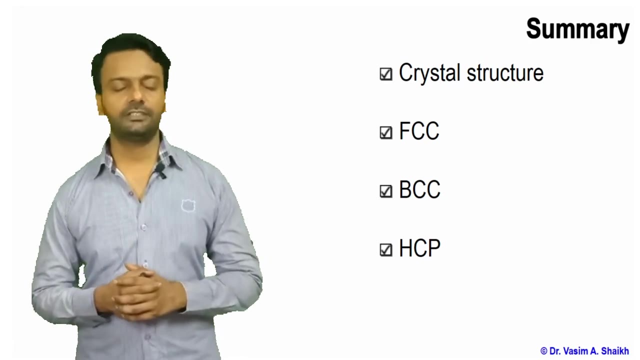 and eight atoms are there in the corner. the atomic packing factor comes out to be 74 bcc c. one atom is in the interior, eight atoms are located in the corner and the atomic packing factor comes out to be sixty-eight percent. in hcp crystal structure we have three atoms which are that in the interior, one atom in the faces. 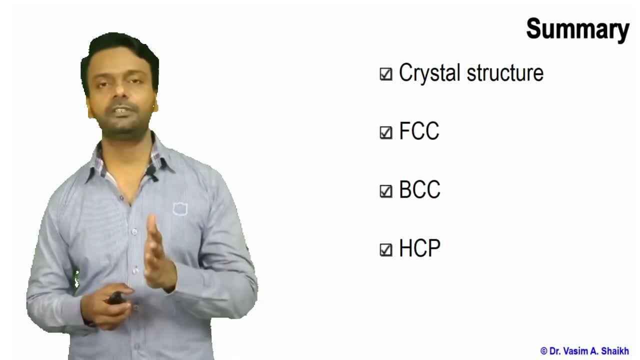 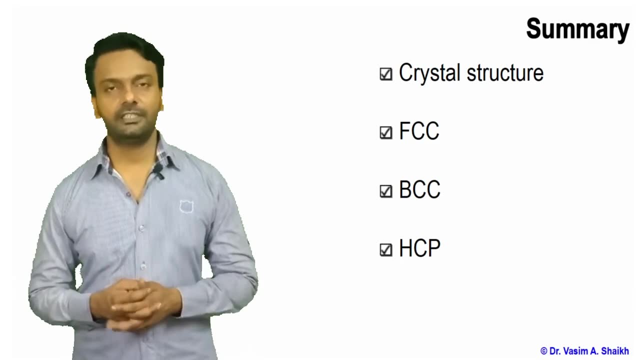 okay, and in the corner we we have two atoms. so 3 plus 1 plus 2 comes out to be 6 atoms per unit cell and the atomic packing factor is same, like FCC is 74 percent. so I hope you like the video and if you really like the 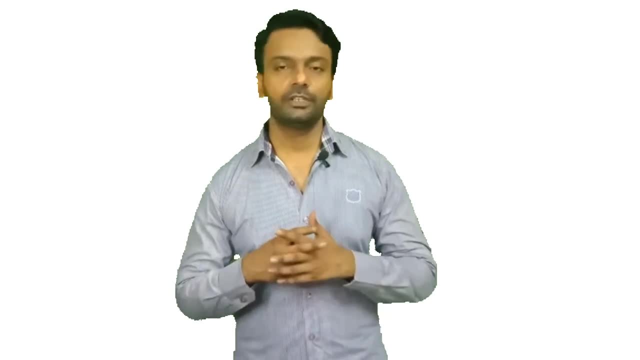 video. you can give it a thumbs up. you can like the video. if you want to listen to more such videos, you can subscribe to my channel. thank you very much. all the best.